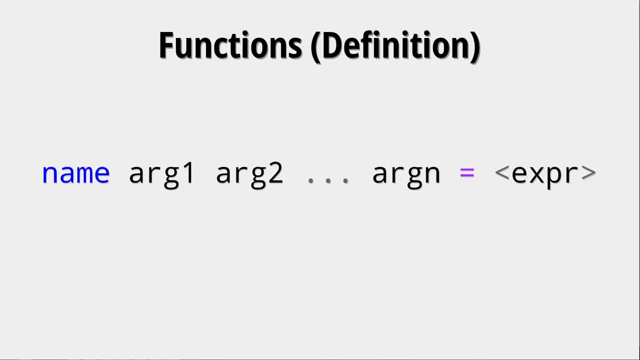 So we do not really have a return like we have in imperative languages. So the expression that a function is defined as is what this function returns. If we look at a function application, this is simply done with writing the name and then the arguments. There are no parentheses and no commas between the arguments and 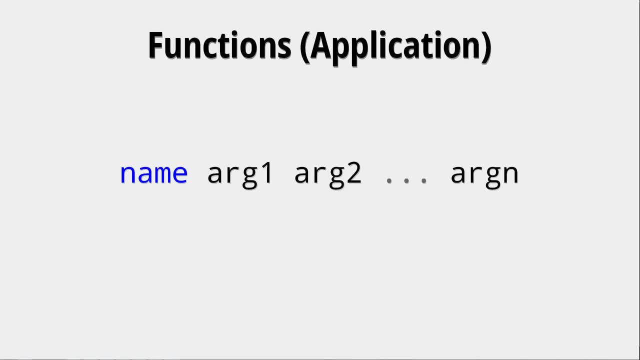 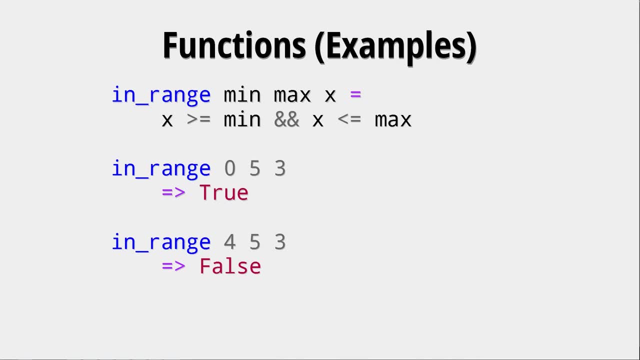 no parentheses around them, because this actually is the syntax for another data type that we will look at in a later video. Okay, so let's look at an example. This in range function: if this x is between min and max- And here we already have the definition of the function- 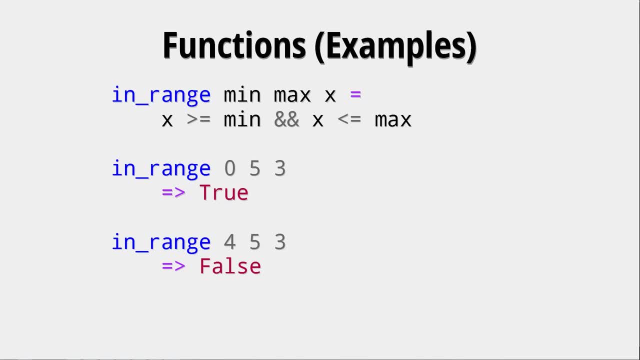 It is defined as well, some composition of other functions. You might say, well, there is some comparison done here and then a Boolean end, which is true. But those comparisons and the Boolean end are actually function calls. They are just written in an infix notation. 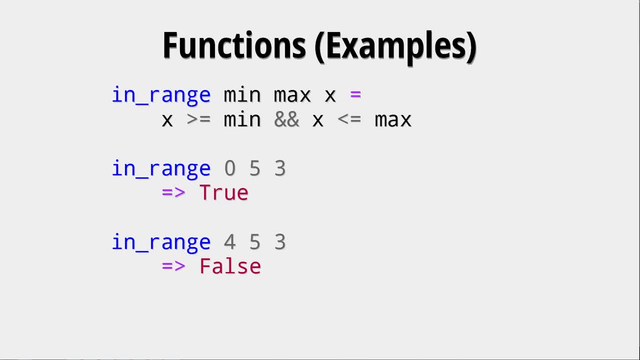 How that infix notation works we will look at in a few slides. It's just very important to see that we do not have something like a return statement. The last expression that is evaluated, or simply the expression that is evaluated, is what we return. So this whole thing. 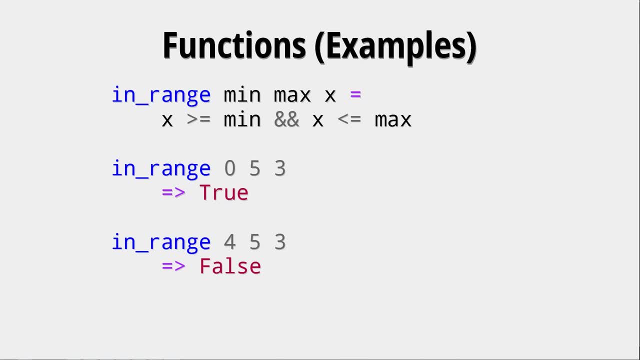 x is bigger or equal to min and x smaller or equal to max. that is what our expression is, And here we can see some applications in range of 0,, 5,- 3 is of course true- and in range of 4,. 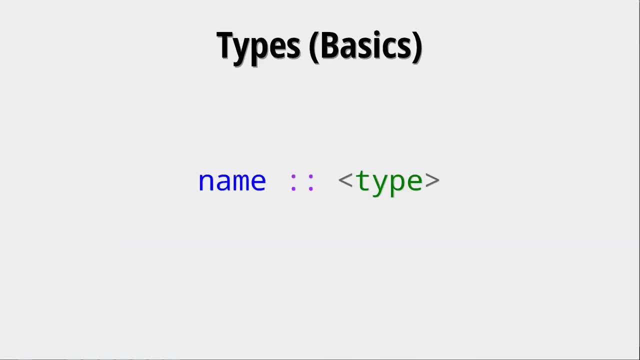 5, 3 is false. Okay, so let's look at types. Every value in Haskell has a type and that type is strict, So let's look at how they are defined. You have the name of your value, then two colons. 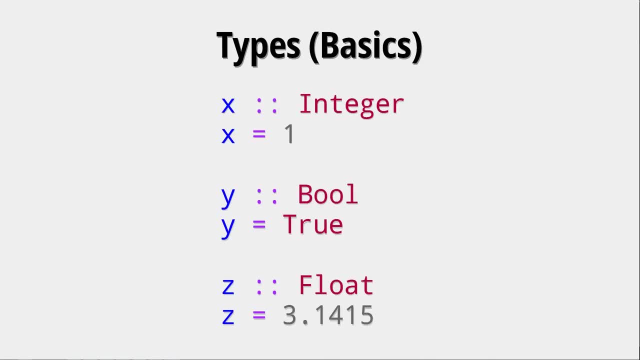 and then the type. So let's look at some examples. For example, here we have the types for x, y and z, which are an integer, a bool and a float. There are many different data types and you should look at them on Haskellorg, for example. 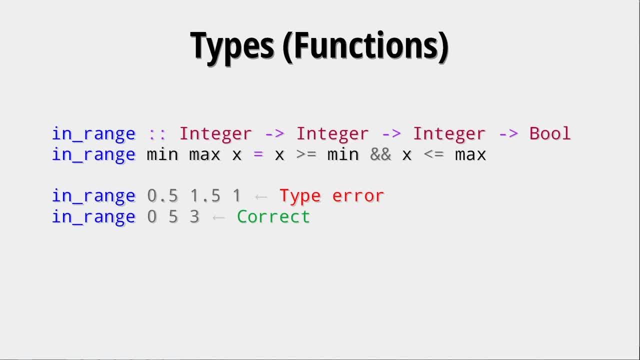 Now functions have their own types, since functions are just values. This is very important, and we will get to that in another video. But let's look at how types for functions work. Well, you basically write them as a list of types for your arguments and then, whatever the type, 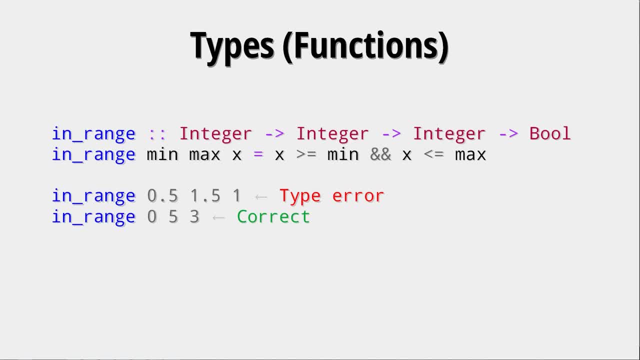 for your return value is. So in this case, we want in range, to get three integers and then return a bool. This is not the only type you could assign to this function. You could also do this with floats, but here, in this case, we do it with integers. It's very important to see that. 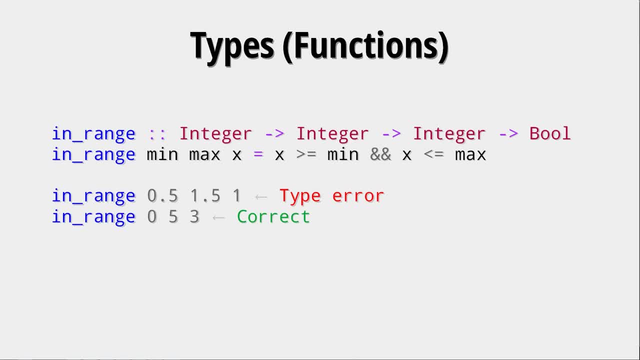 for example here: if you call this function with floats, it will return a type error. It will not return anything, it will just produce a type error. But of course it works with integers. Now sometimes you want to do something like this, where you save the result of some expression in a. 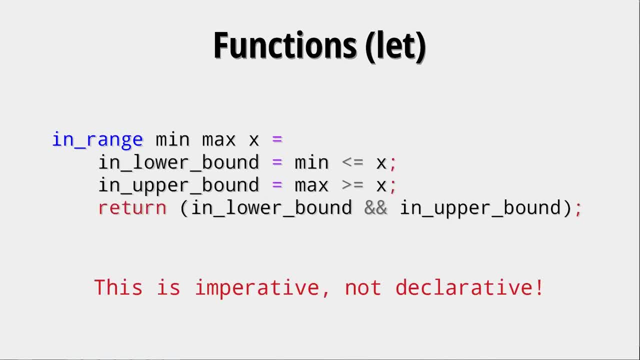 variable and then return a type error. So let's look at how types for functions work. Well, an end statement. Of course, this would be imperative and not declarative. This is also not proper Haskell syntax. So the question is: how can we do something like that? And we can do it. 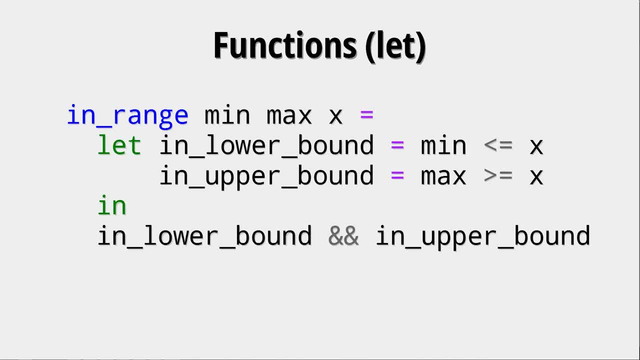 with so-called let bindings, where we bind the result of some expression to a name, like in lower bound, and then produce an end result, the last expression, so to speak, in relation to whatever names we just defined. And then we can do something like this where we bind the result of some 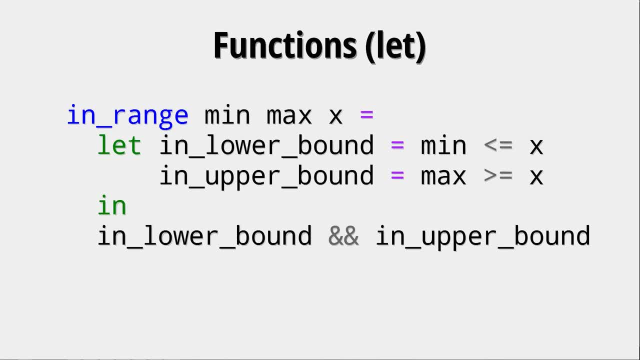 name, like in lower bound, and then produce an end result, the last expression, so to speak, in relation to whatever names we just defined. It generally works like this: that we say: let then some name equals some expression, and then maybe some other names and other expressions in, and then the final. 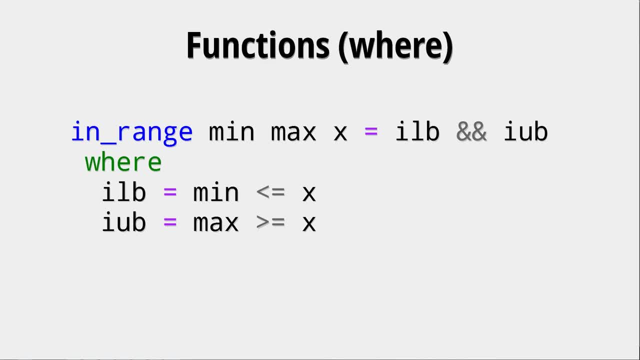 expression. Another way of doing this is with a where binding, where you have the final result of your function And in the end say where you know certain names are defined as certain expressions. Again, it's very important to see that in the example of the let binding.